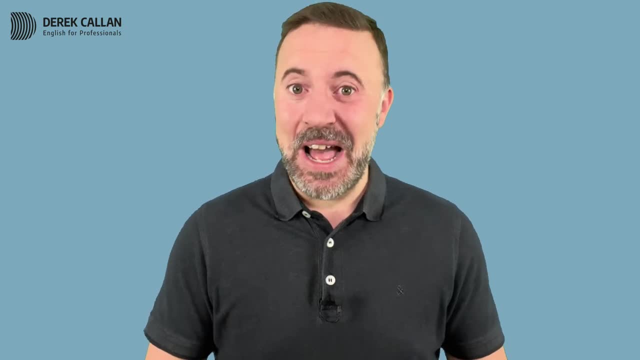 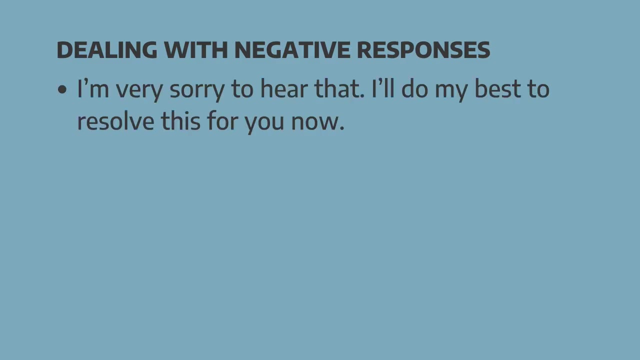 answer the call and greet the customer. sometimes they have a problem that they want to tell us about. here's what we can say. i'm very sorry to hear that. i'll do my best to resolve this for you now, or? i'm so sorry to hear that, if you could give me your name and order number, 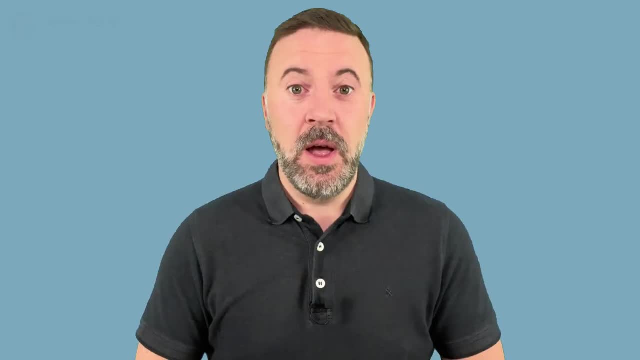 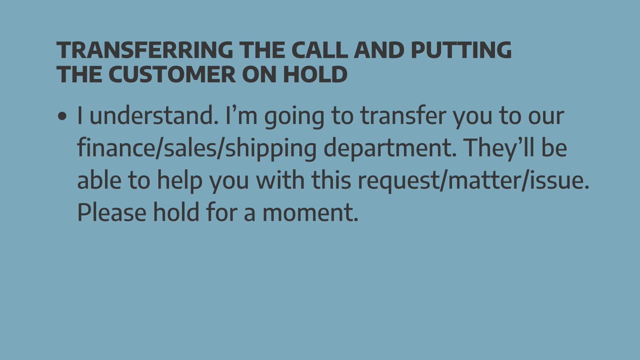 i'll start looking into this immediately. but what if you're not the right person to help the customer? you may need to transfer them to a different person or department. i understand i'm going to transfer you to our finance or sales or shipping department. they'll be able to help you with this. request matter issue. please hold for a moment or. 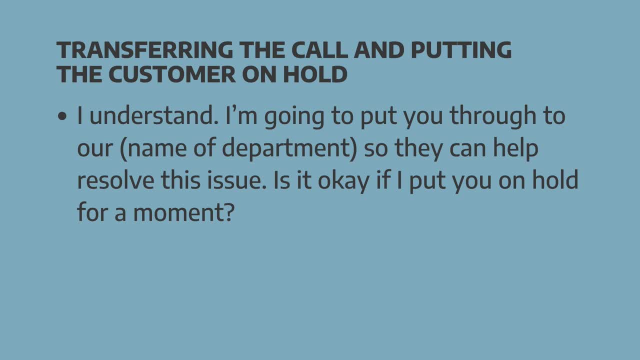 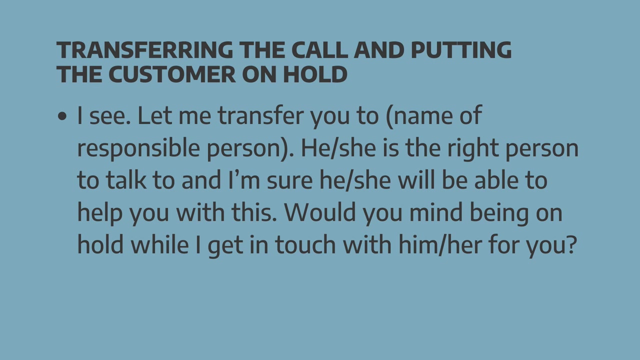 i understand. i'm going to put you through to our name of department so they can help resolve this issue. is it okay if i put you on hold for a moment? or? i see, let me transfer you to name of responsible person. he or she is the right person to talk to and i'm sure he or she will be able to help you. 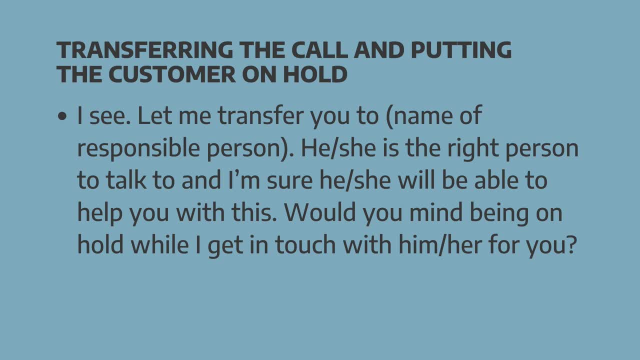 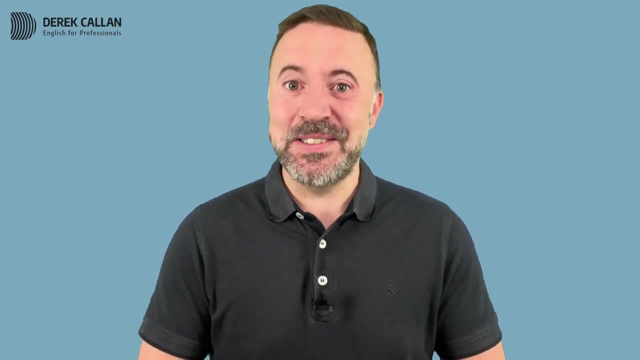 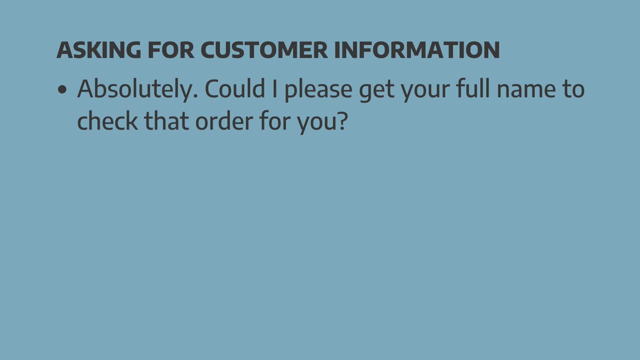 with this. would you mind being on hold while i get in touch with him or her for you? if you are the right person to help the customer, you'll probably need to get some customer information from them, absolutely. could i please get your full name to check that order for you? 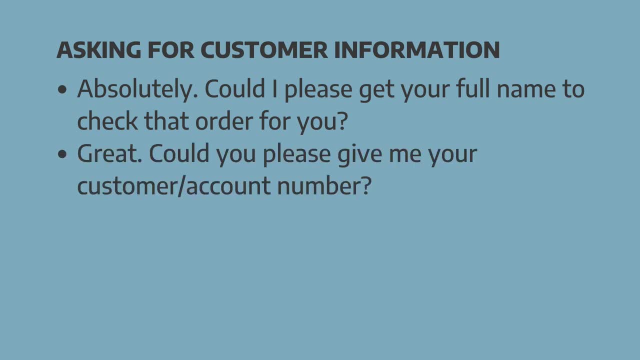 or great. could you please give me your customer or your account number? no problem, do you happen to have the order number so i can bring it up? do you happen to have? is just slightly more friendly and polite than saying do you have? and to bring something up means to bring it up on a screen. 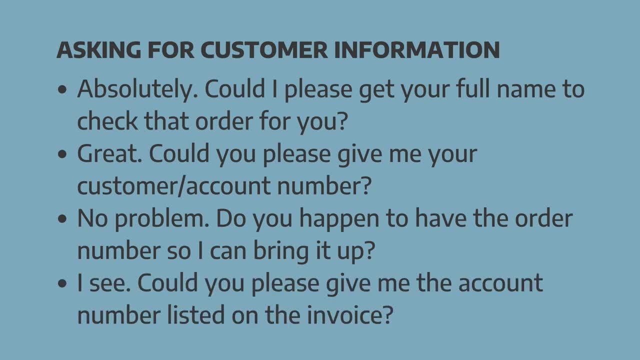 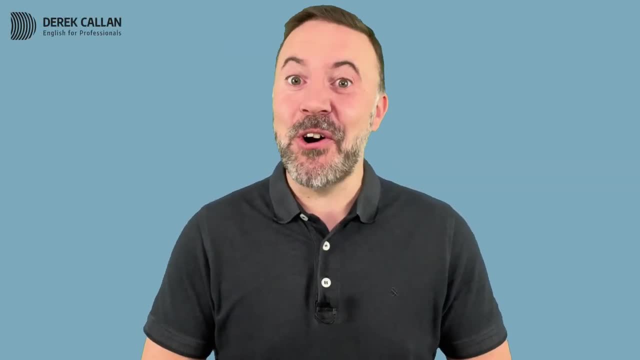 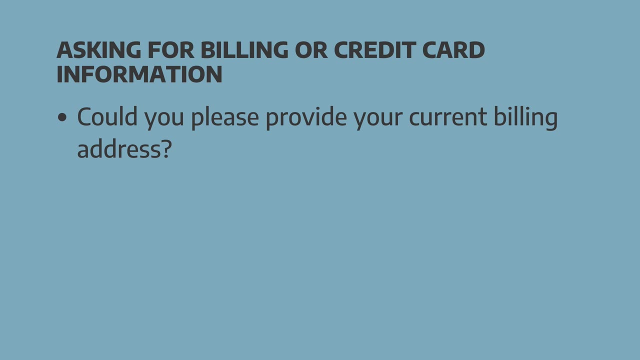 in front of you, i see. could you please give me the account number listed on the invoice, and you might also need to ask the customer for billing or credit card information. could you please provide your current billing address or could you please verify your address? could i please have your credit card number? cvv code. 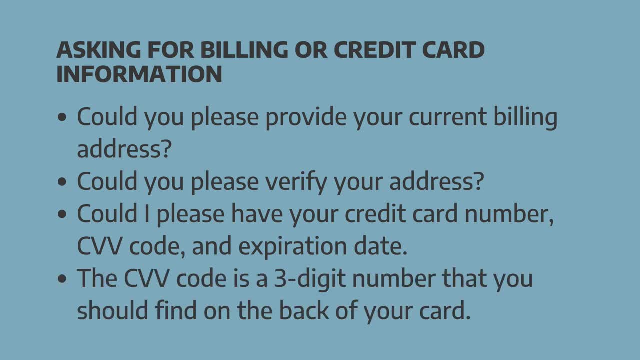 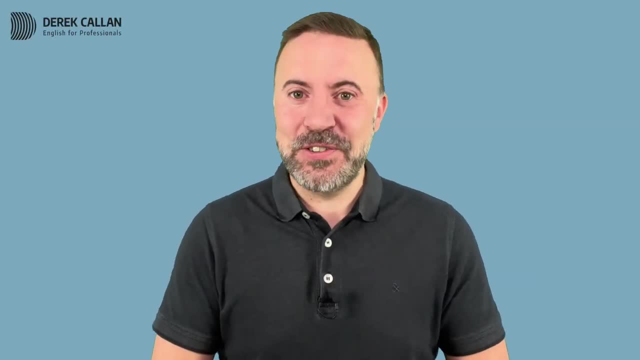 and expiration date. the cvv code is a three digit number that you should find on the back of your card. when dealing with customer requests or questions, we often need a few minutes to check or find other information. here's what we can say in this situation. i see i'm going to need a moment. 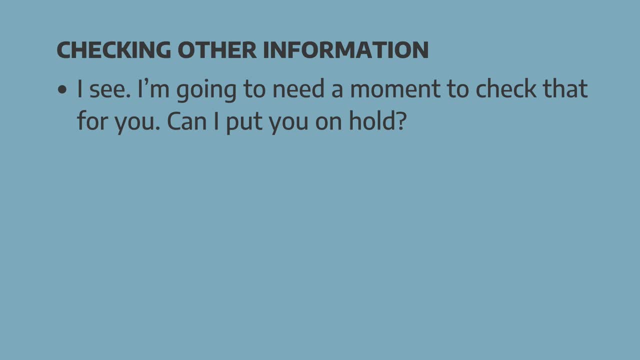 to check that for you. can i put you on hold, or i understand? please give me a minute while i pull up that information. would you mind being on hold while i do that? to pull up information is very similar to bring up, to pull it up on the screen in front of you If we ask the customer to. 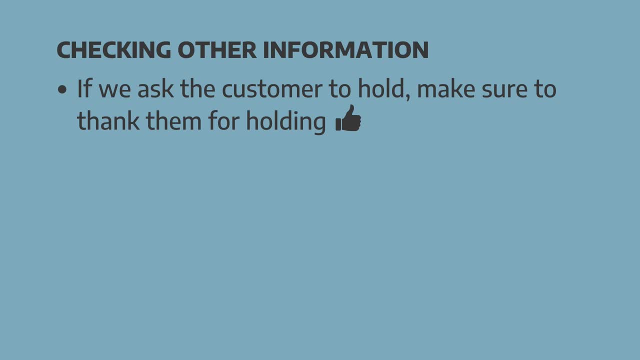 hold. it's very important to thank the customer for holding once we're back on the call with them After checking the information, it's very common to say the customer's name like a question to make sure they're still on the line, then say thank you for holding. I have that information for you now. 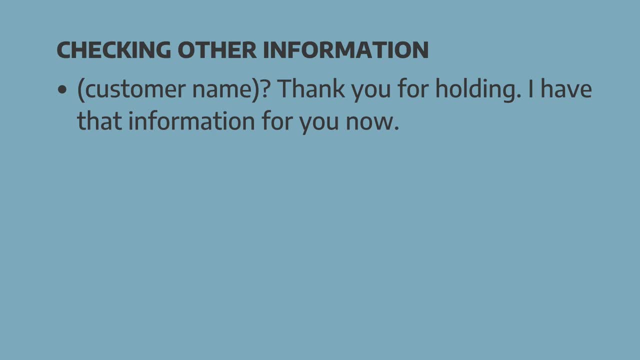 For example: Mr Callan, thank you for holding. I have that information for you now. Or Mr Callan, thank you for holding. I'm sorry, it took a little longer than expected. Or, Mr Callan. 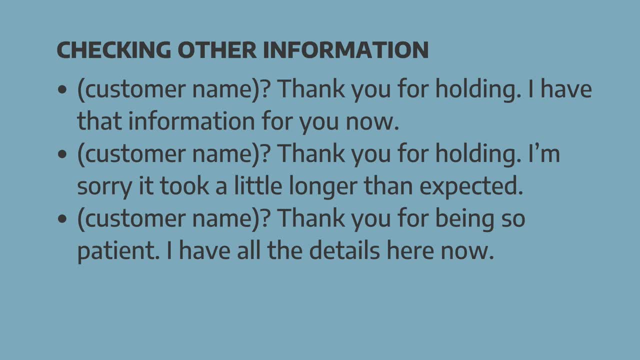 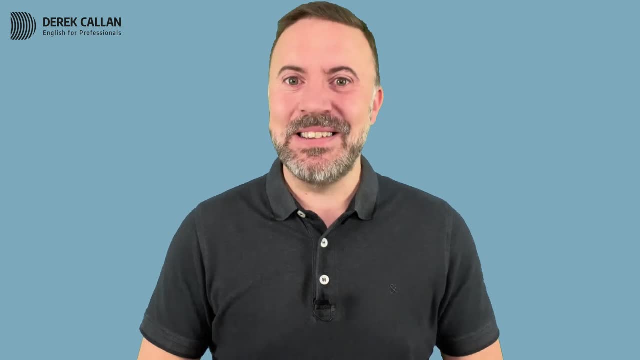 thank you for being so patient. I have all the details here now, And now it's time to move on to the unpleasant part: dealing with problems, complaints, issues. And here's a tip for you: If there is a problem, there's a way to solve it. If there is a problem, there's a way to solve it. 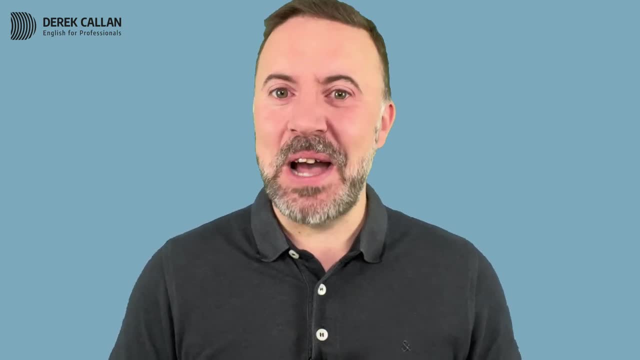 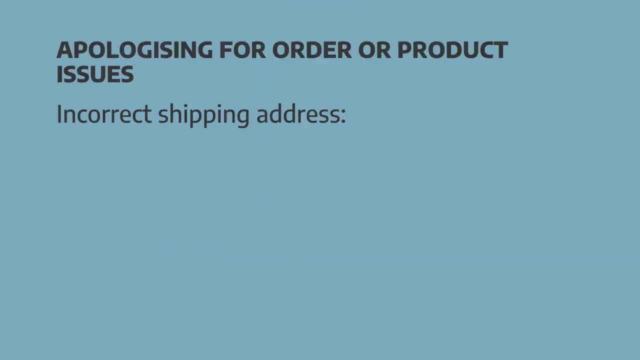 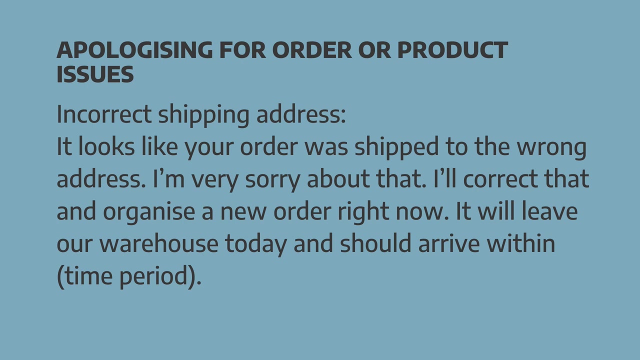 If there is a problem or issue of any kind, it doesn't matter whose fault it is. always show understanding for the customer's situation. And our first example is incorrect shipping address. It looks like your order was shipped to the wrong address. I'm very sorry about that. I'll correct that and organize a new order right. 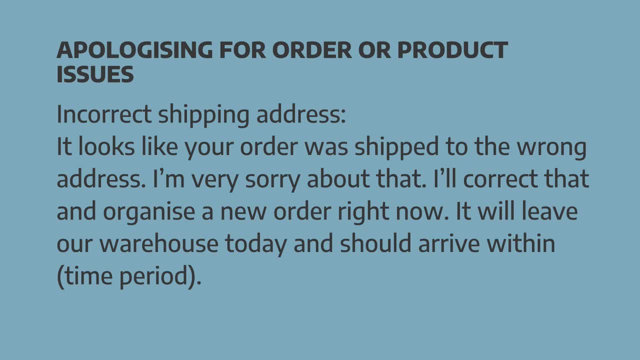 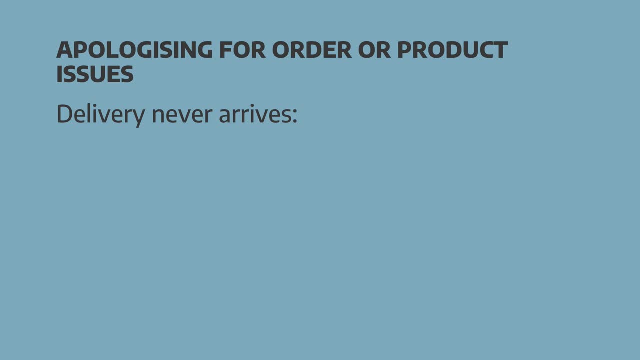 now. It will leave our warehouse today and should arrive within and then give the time period. Example. Example two: the delivery never arrives. I'm so sorry to hear that. And then use the customer name. Let me bring up your order so we can see what happened and make sure that delivery arrives. 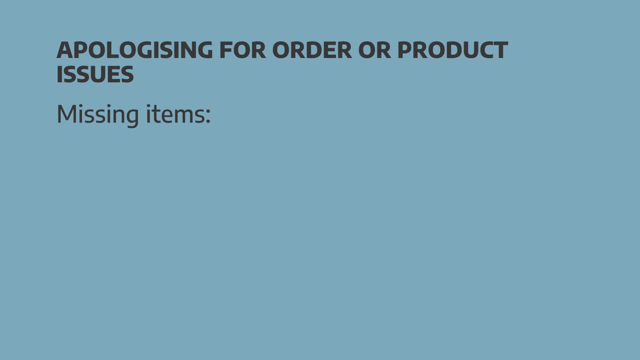 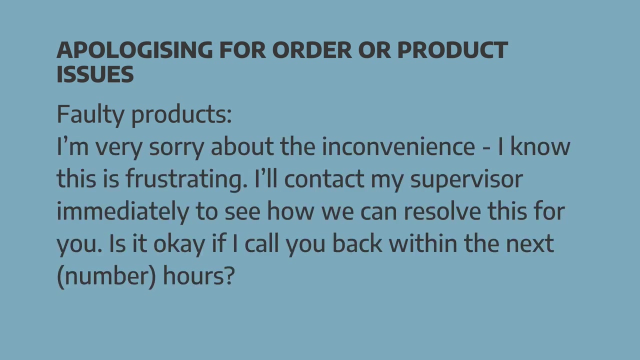 this time. Example three: missing items. I'm so sorry about this mix-up. I will correct the order and get the missing items to you as soon as possible. Example four: faulty products. I'm very sorry about the inconvenience. I know that the delivery never arrives. I'm so sorry about this. 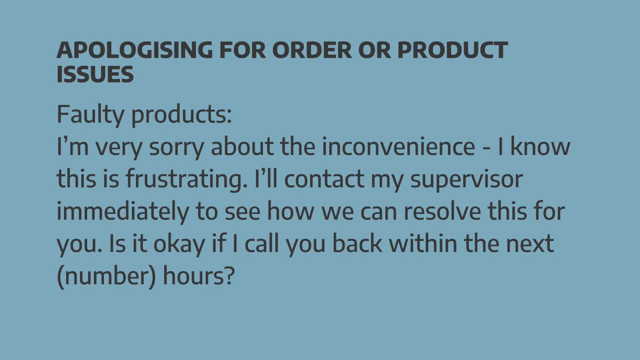 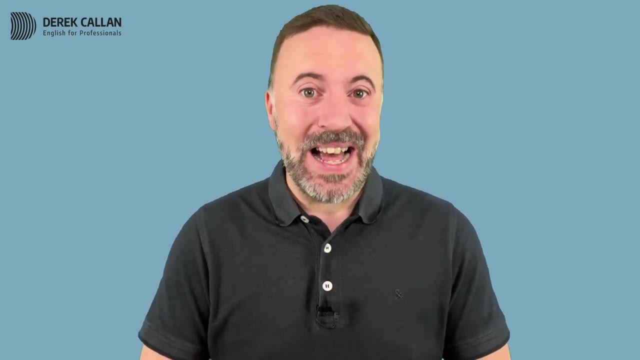 mix-up. I'll contact my supervisor immediately to see how we can resolve this for you. Is it okay if I call you back within the next and then say the number hours? Sometimes when there's an issue or a problem, customers can get quite angry or impatient. It's important to stay professional. 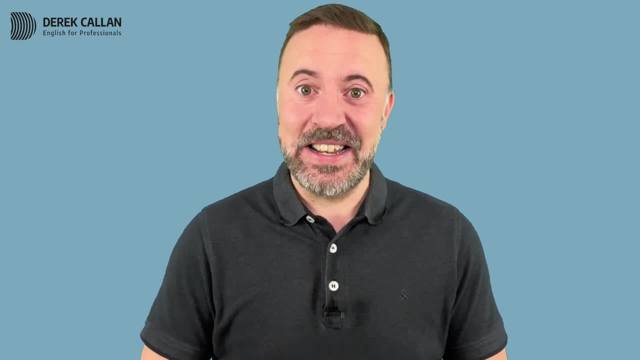 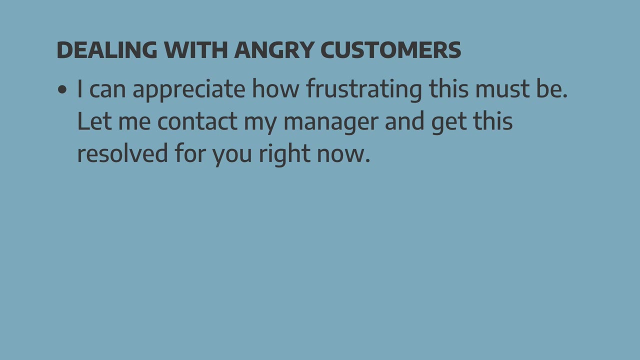 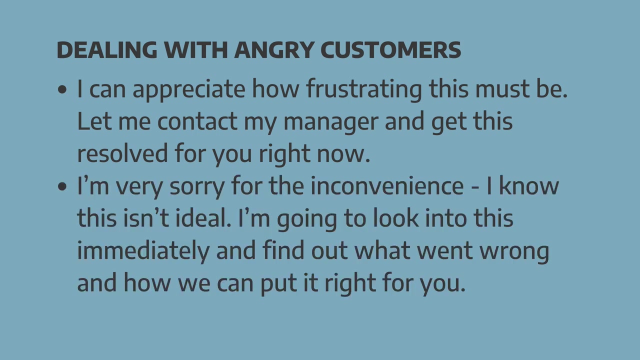 and calm and again, to show understanding. I can appreciate how frustrating this must be. Let me contact my manager and get this resolved for you right now, Or I'm very sorry for the inconvenience. I know this isn't ideal. I'm going to look into this immediately and find out what. 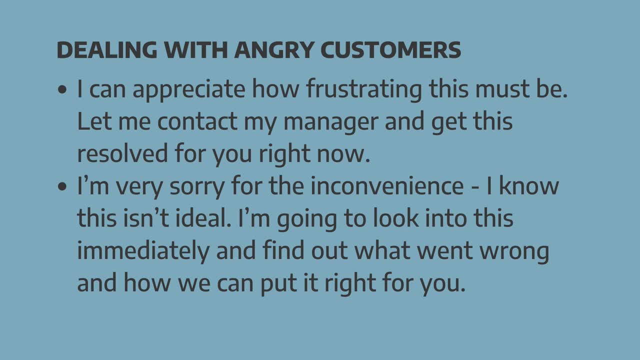 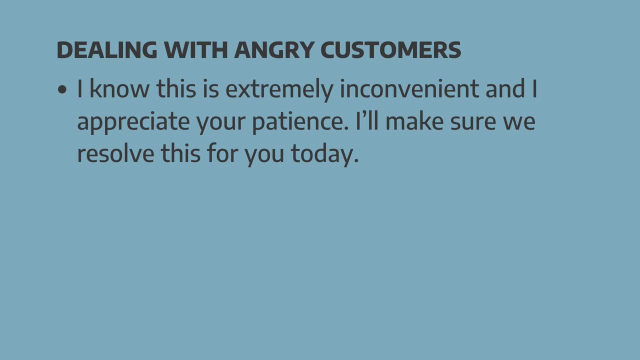 went wrong and how we can put it right for you. Or- I know this is extremely inconvenient and I appreciate your patience- I'll make sure we resolve this for you today, Or I'm going to do everything I can to get this resolved as soon as possible. And one more example: I totally 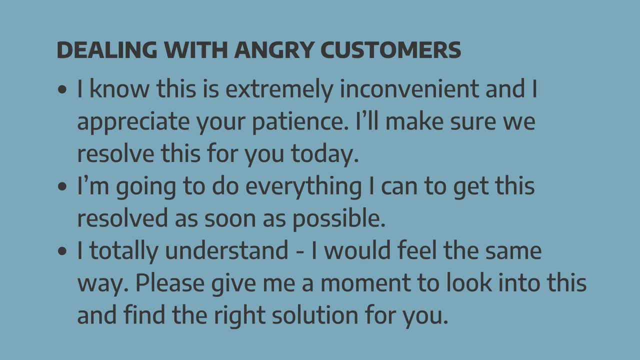 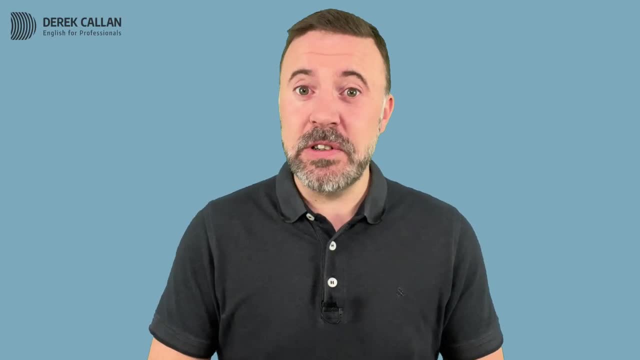 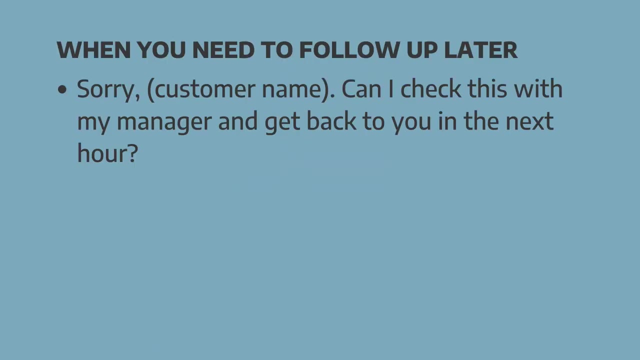 understand. I would feel the same way. Please give me a moment to look into this and find the right solution for you. But what if we can't fully resolve the issue for the customer on that call? What do we say Sorry and then use the customer's name? Can I check this with my manager and get? back to you in the next hour Or I'm very sorry for the inconvenience. I know this is extremely inconvenient. I know this is extremely inconvenient, But what do we say Sorry and then use the customer's name? Can I check this with my manager and get back to you in the next hour? Or I'm very 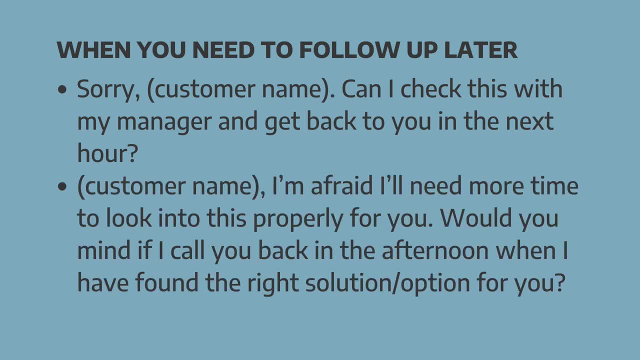 sorry for the inconvenience. I know this is extremely inconvenient, But what do we say? Sorry and then use the customer's name- Can I check this with my manager and get back to you in the next hour- Or customer name. I'm afraid I'll need more time to look into this properly for you, Would you? 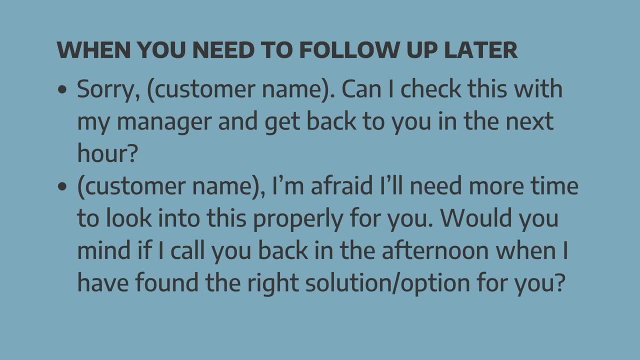 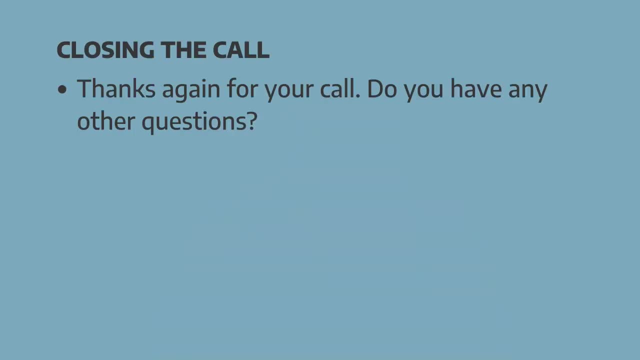 mind if I call you back in the afternoon when I've found the right solution or the right option for you. And here are some different ways to close the call. Thanks again for your call. Do you have any other questions? Or well, I'm glad I could help you resolve this issue. Is there anything?